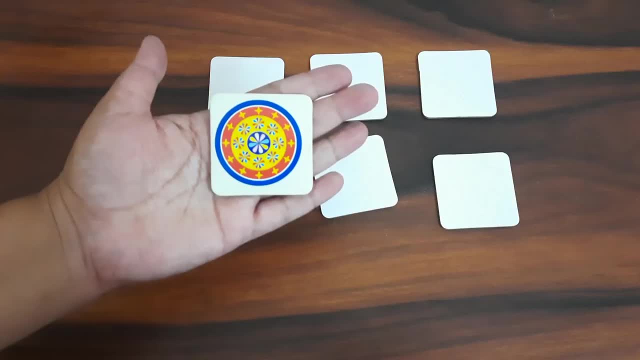 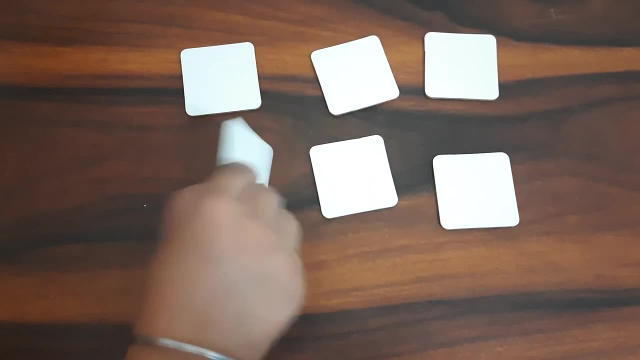 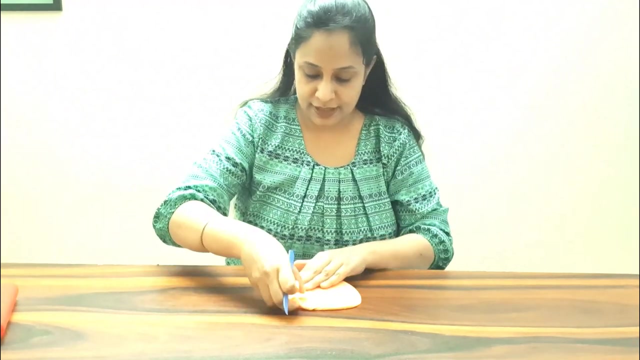 and then trying to recall generally what the items were. or you can simply ask them to look at a card, turn it around and ask them what the card was, or try to find it in an array. putty is very good and I love it for getting the children learning the concept of letters. 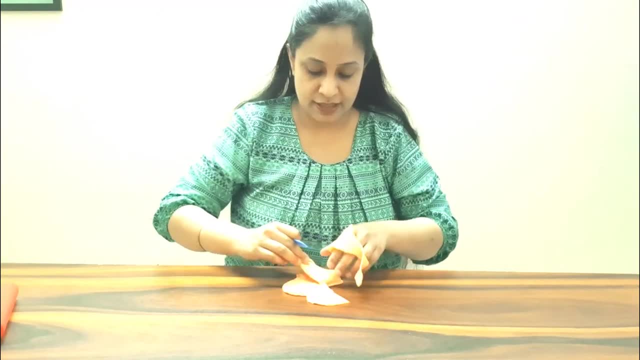 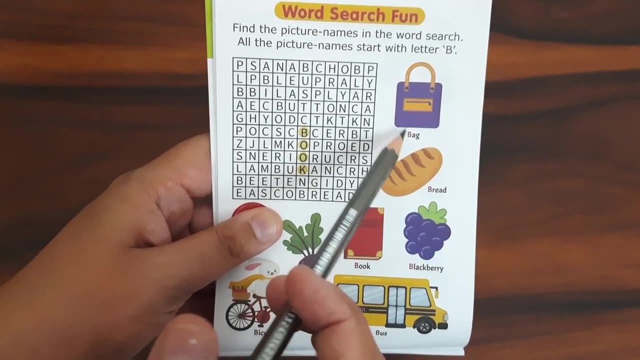 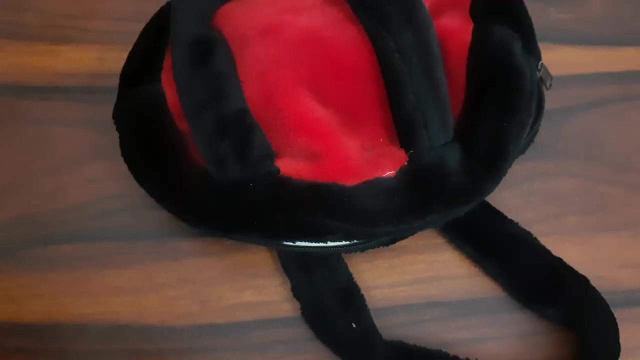 numbers shape and you can check out my video for how putty is so important in pre-writing skills. word search is a very good activity that the child can perform where there is a random array of letters from which they have to try to find some words. a stereognosis game is. 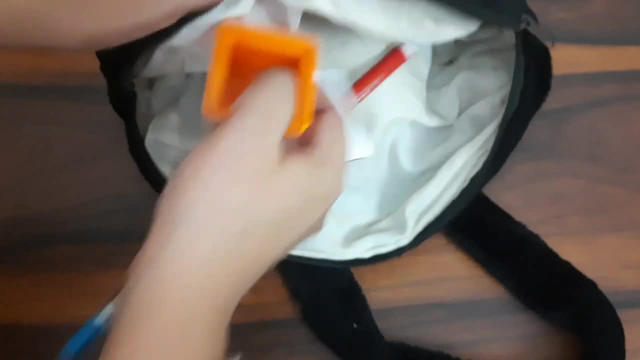 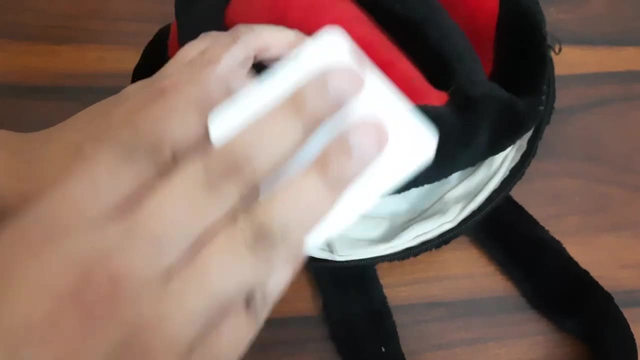 going to do wonders for them, where the child, simply by touch, has to find objects in a bag. so, for example, you place their known items in a bag, letting them touch and feel it, and then placing them in a bag and trying to tell them to find it without looking, so that their 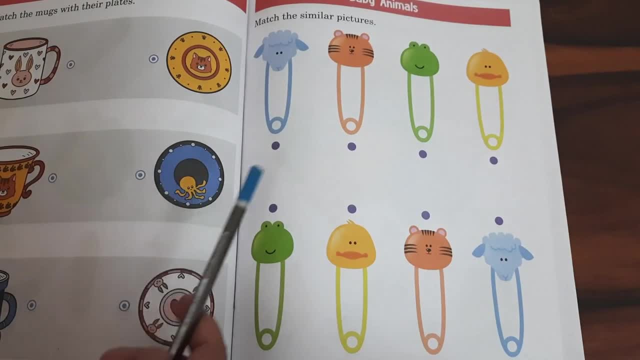 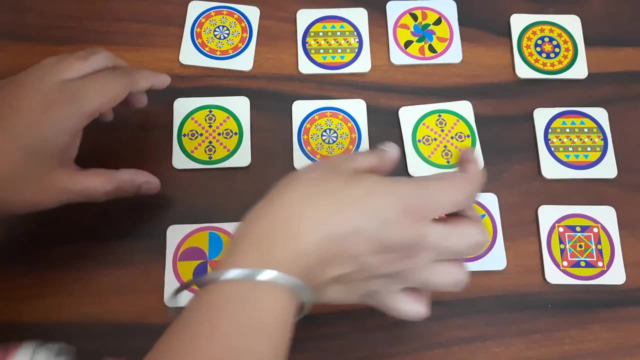 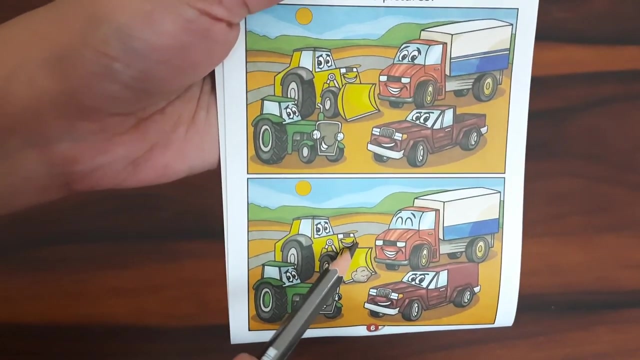 other senses also can see it, and then you can try to find it without looking, so that their other senses also get heightened. matching activities are an excellent form of visual perception, in which you match the cards, or you show them one card and then they try to find it in an array, or simply trying to find difference between pictures. that also help. 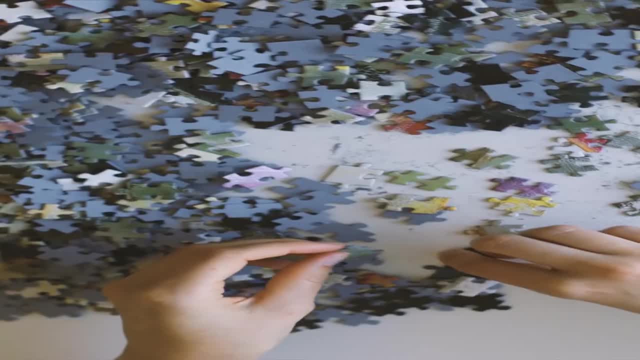 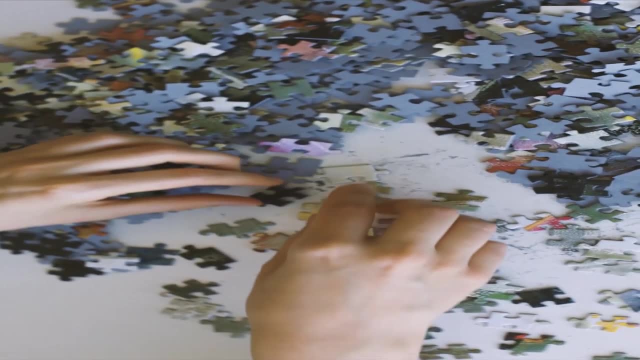 so increasing the number of differences as you go. and finally, jigsaw puzzles are an excellent way in which you can keep increasing the number of pieces that they have to pick up as you go along with the game. so that's all for today, and I'll see you in the next chapter of the 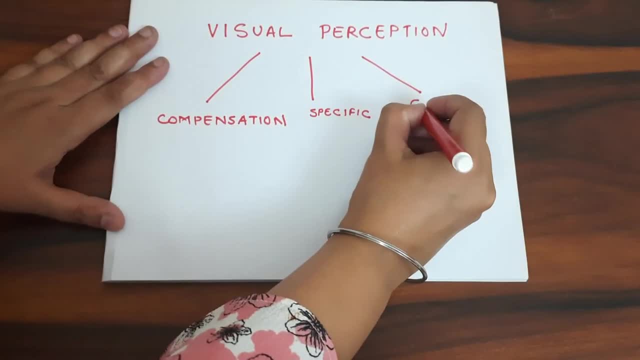 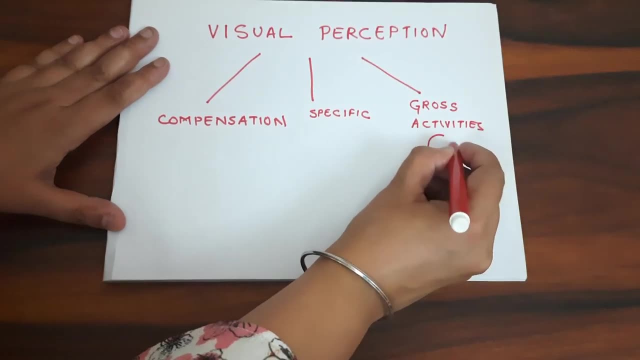 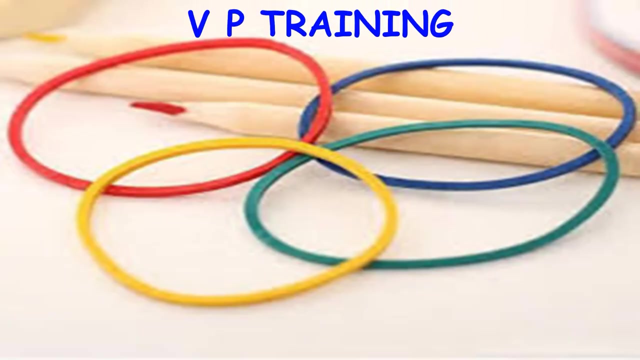 video. see you then, bye, bye, put together. always try to engage your child in activities which are more gross, like playing with the ball, catch, throw, kick, putting a bit in a target like a basketball game, or even riding a bike. these are very simple activities that can help your child in improving their visual perception. 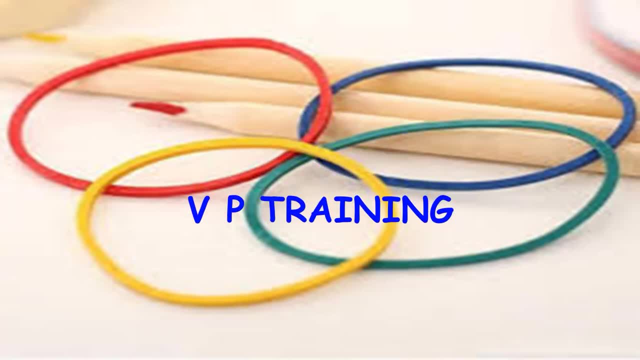 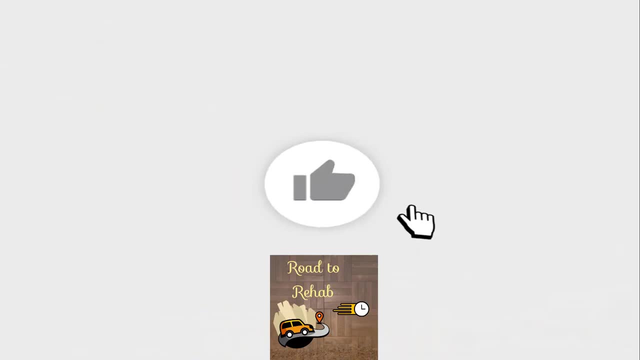 and, in general, should be used by all parents so that the child never faces a problem, either academically or in their daily routine, or even in play. let me know how informative this video was. leave it in the comments below. let me know any other topics that you want me to cover. in the road to rehab channel. we will meet again.